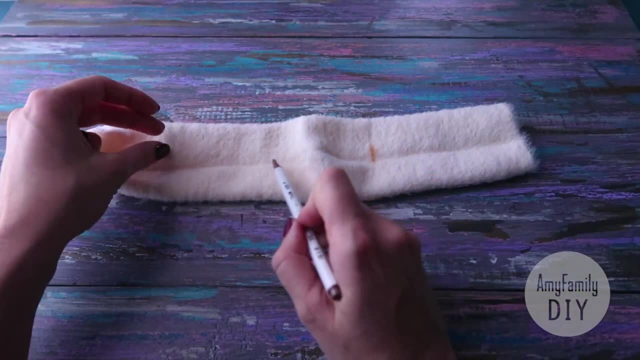 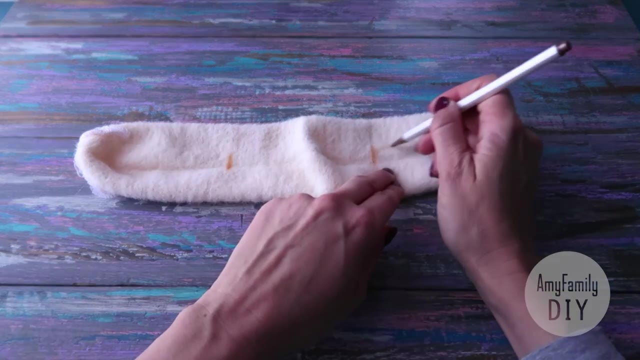 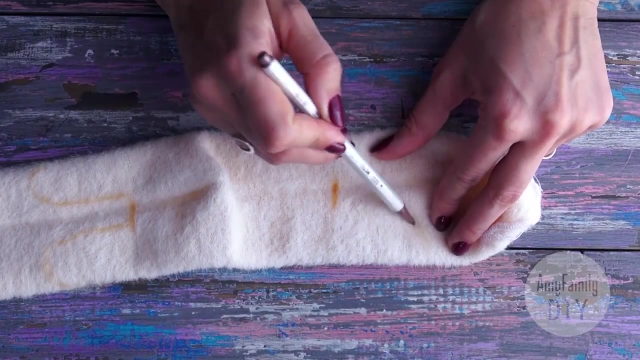 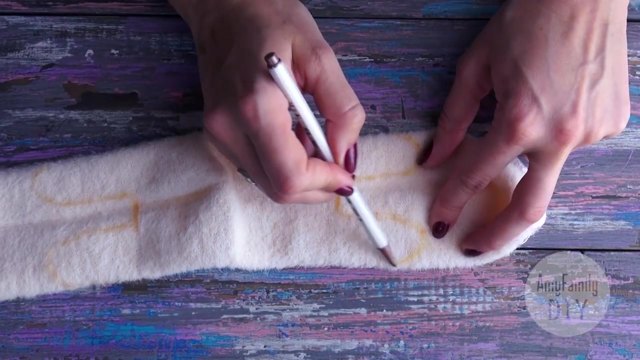 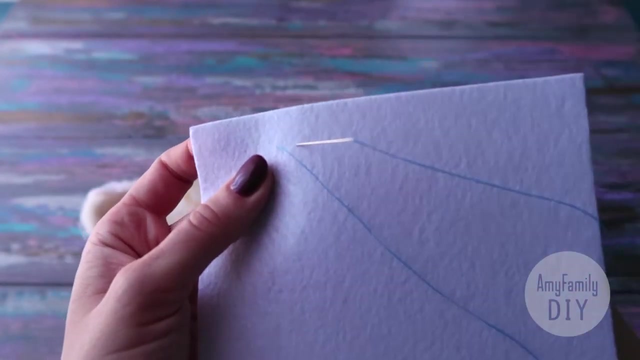 Now I grab my highlighter and draw the paws. The distance to the front paws is a little shorter than to the back ones. And now a brief lyrical digression about the seam we're going to use. It's the most basic classic back stitch. I make the first stitch, pull the needle out a bit. 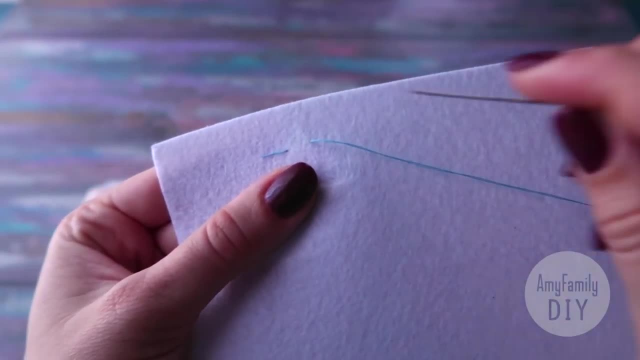 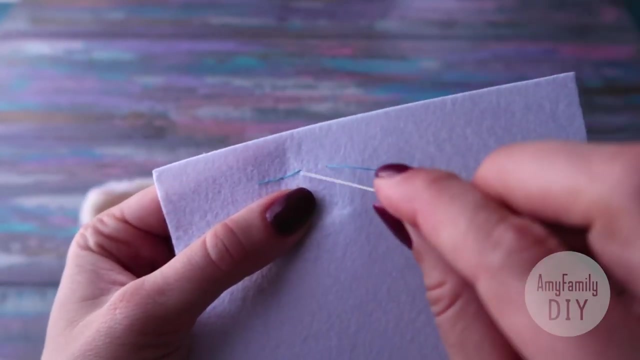 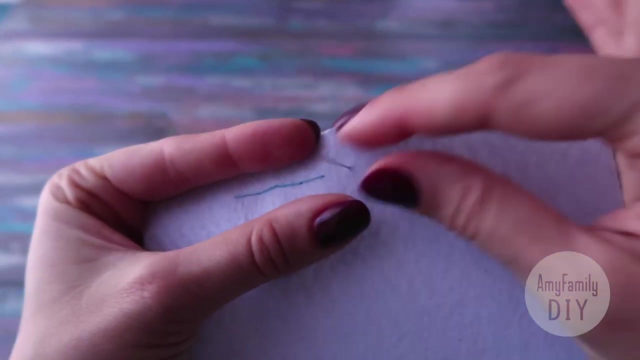 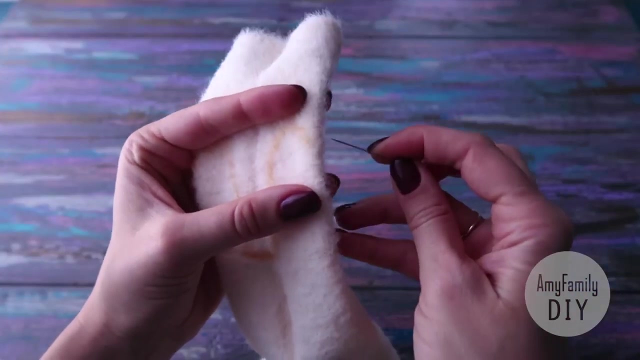 in front and return backwards Again, come out a bit in front and go back. Quite easy, isn't it? This is what the seam looks like on the reverse side. I use the same seam following all the lines I've drawn First, the front paws. 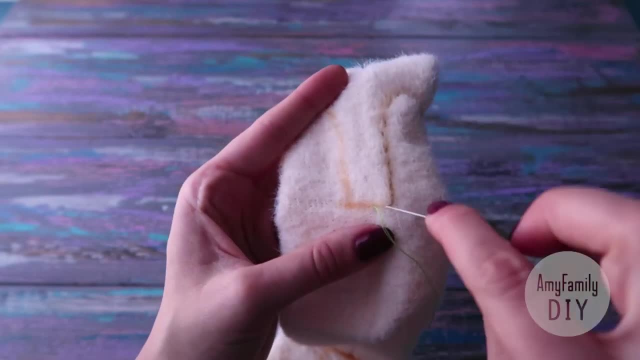 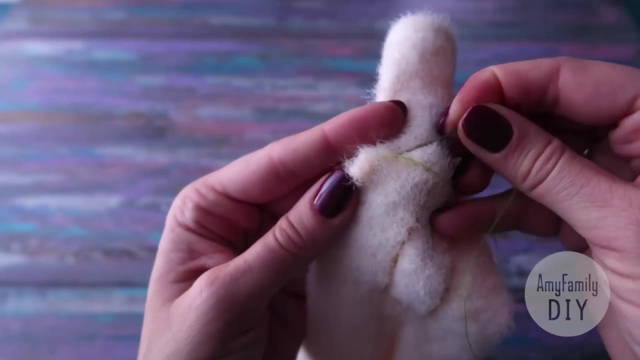 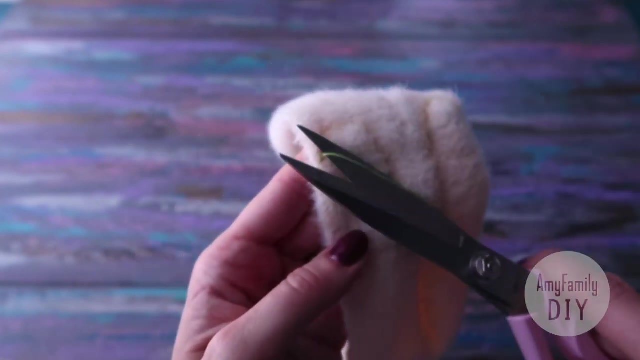 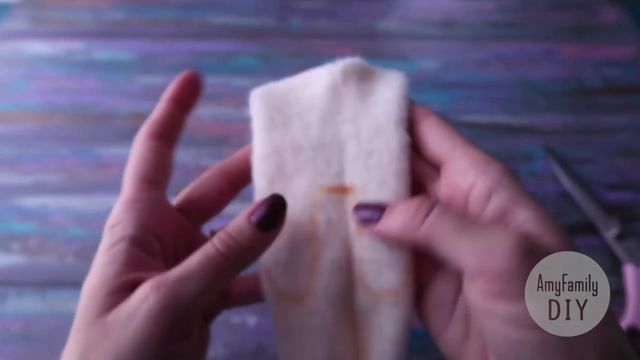 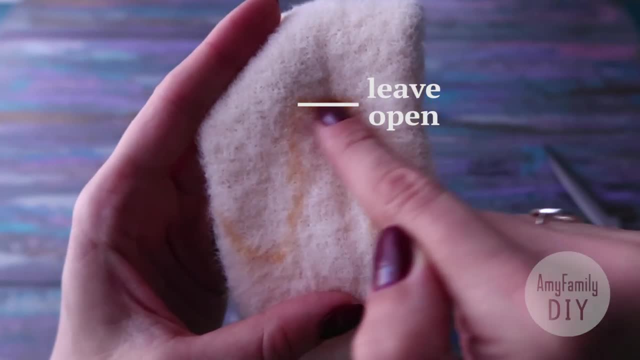 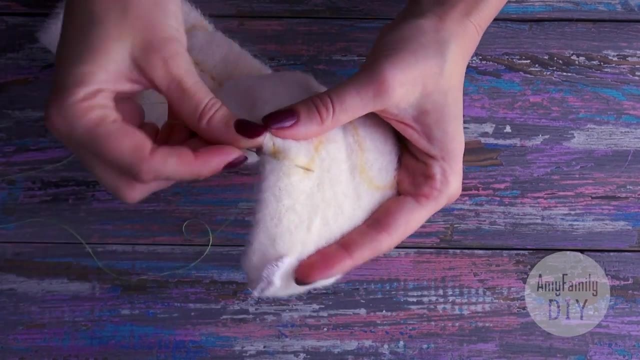 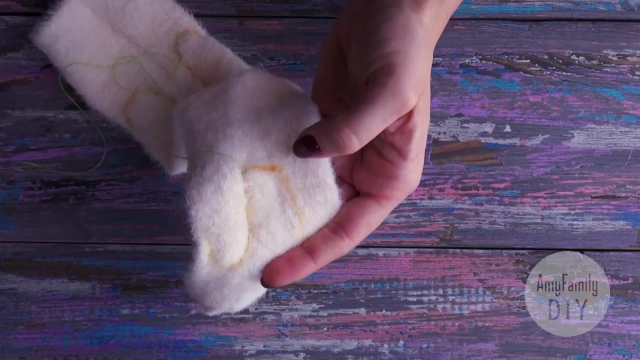 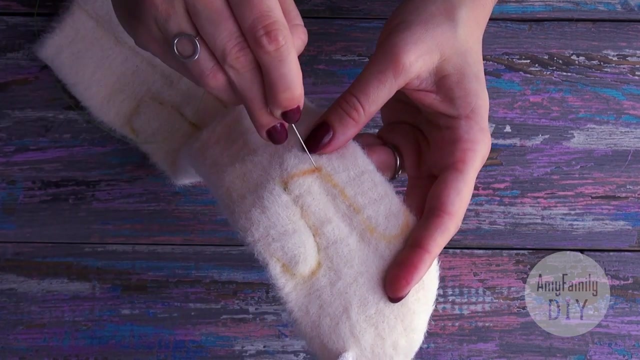 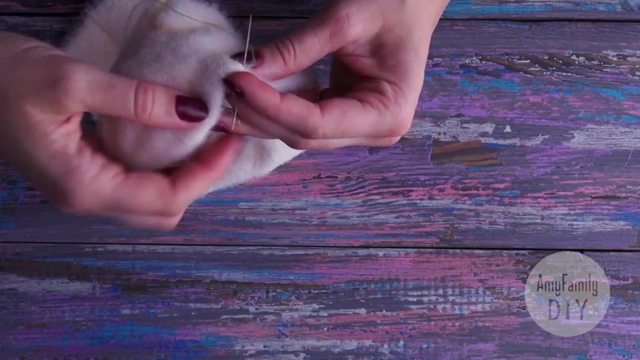 And here we will have to leave a small opening to turn the piece inside out. later Sew along the paw lines, but leave this part open. Do the first paw and cut off the thread, Skip the opening and do the second paw. Now I cut out the kitten's body, leaving a 0.5cm allowance. 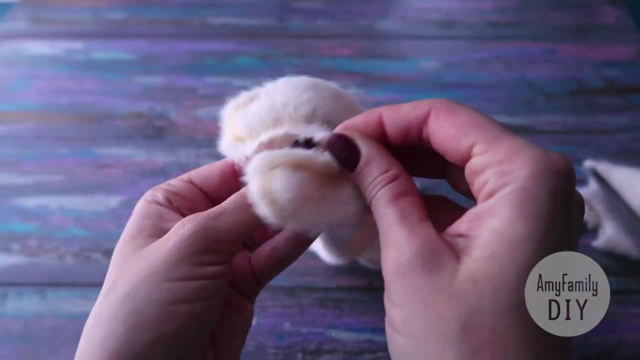 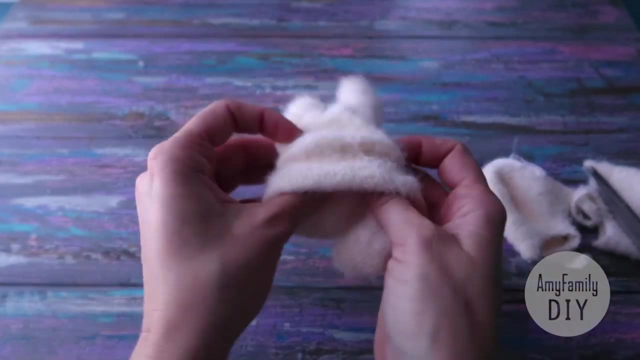 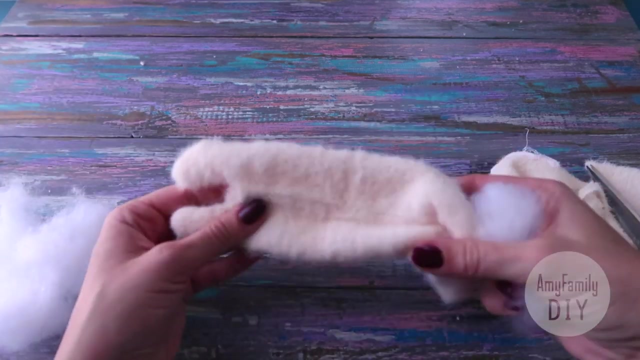 And I turn the piece inside out for the opening. And I turn the piece inside out for the opening. Now, let's grab the stuffing for toys and get down to it. Now, let's grab the stuffing for toys and get down to it. First thing, stuff the paws with small pieces of holofiber. 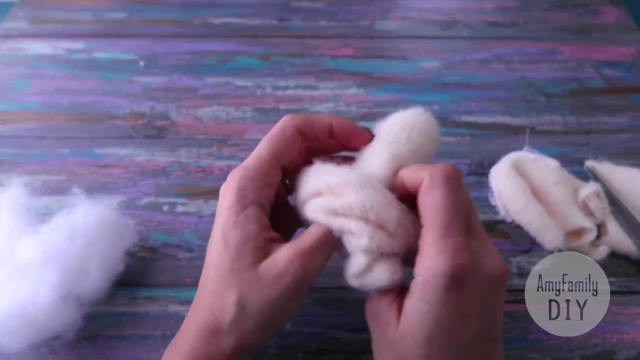 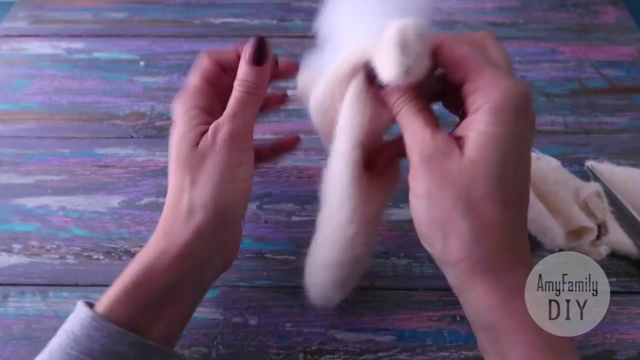 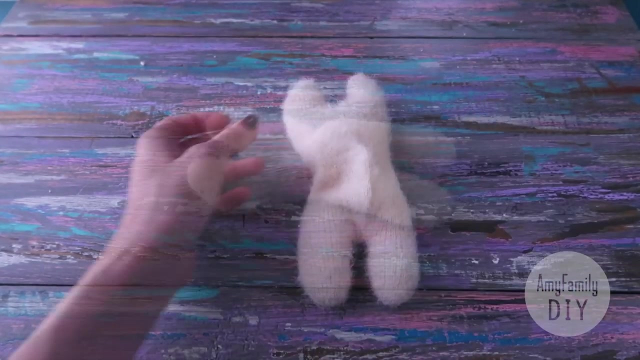 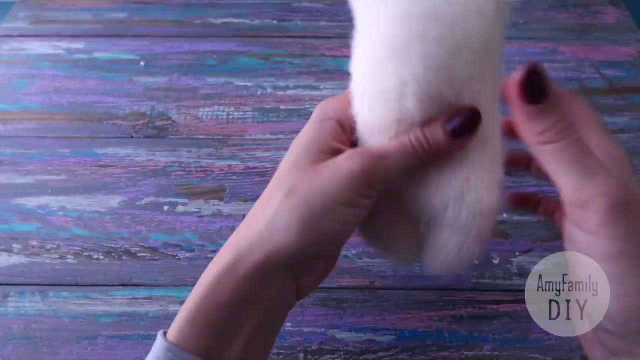 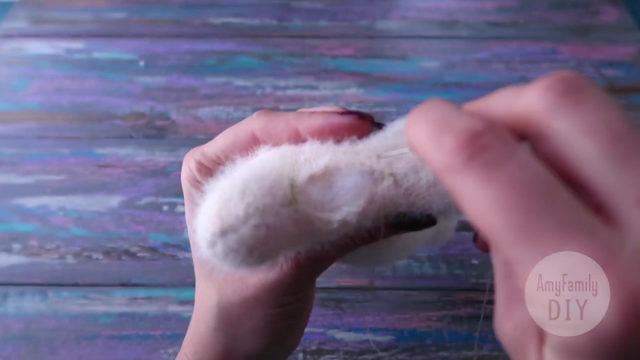 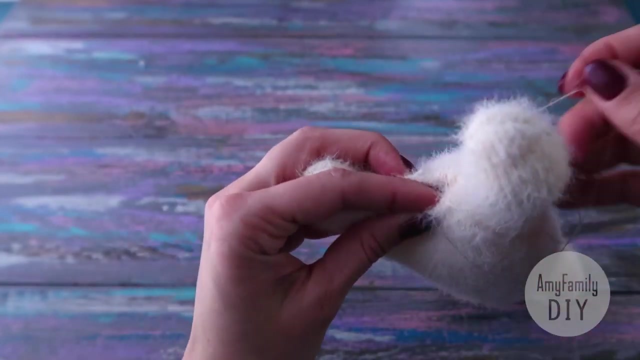 First thing, stuff the paws with small pieces of holofiber, Then stuff the body. Once everything is ready, close the opening. I do it using the invisible stitch that I've already shown you many times. Turn the needle through the fabric of the top and the bottom edge. alternatively, 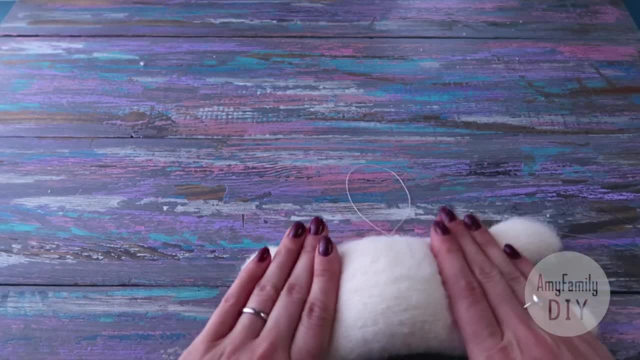 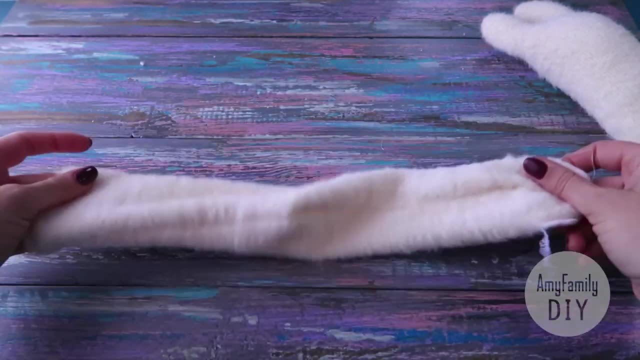 This is the soft body you should eventually get. Let's move on. We will use the second sock from the pair to make the kitten's head Same as in the previous case: turn it inside out and place it in front of yourself, heel. 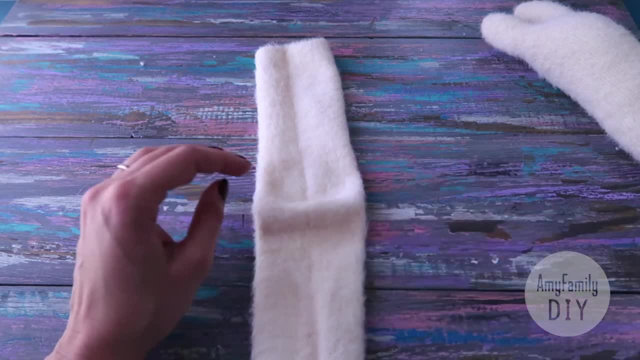 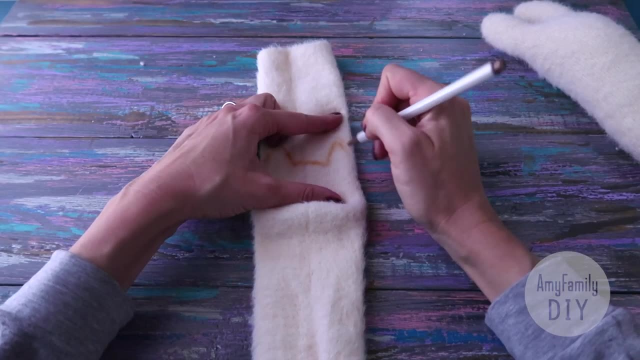 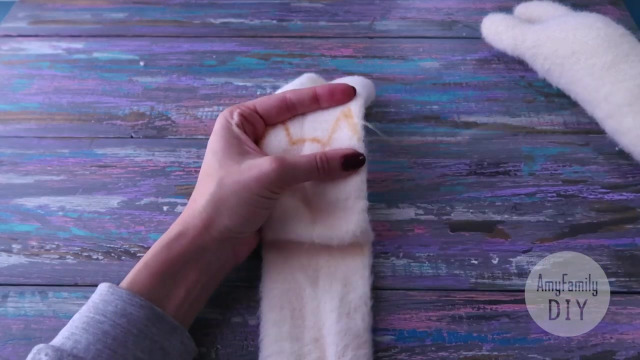 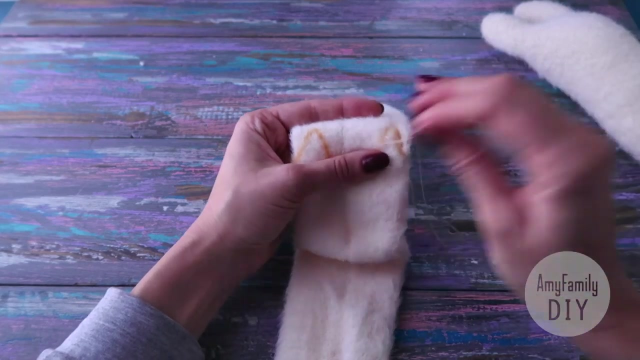 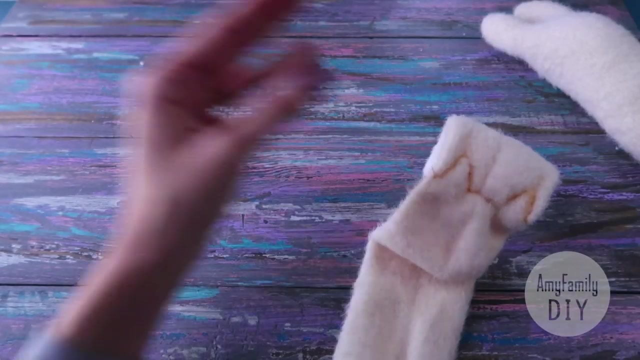 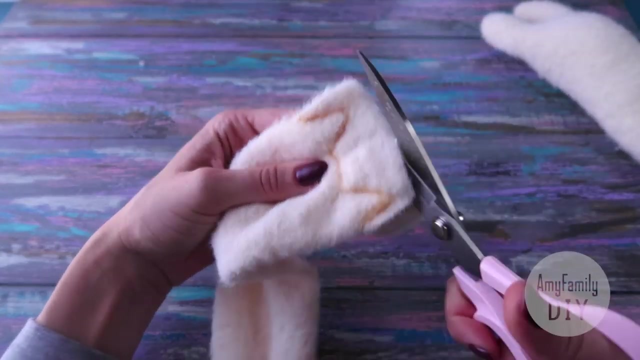 up. The heel will be the kitten's nose. Draw the ears on top like this. Grab your needle and thread and sew along the contour using the backstitch. At this stage, this is what you get. I cut out the piece, leaving half a centimeter allowance. 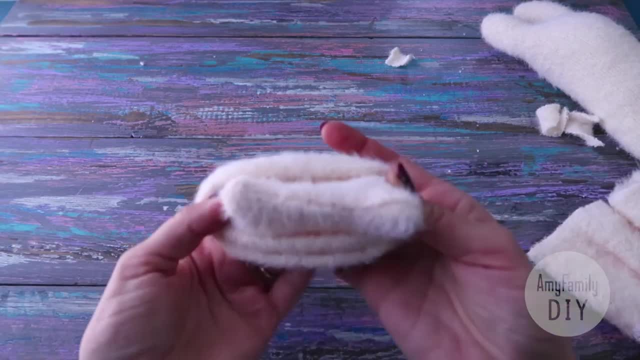 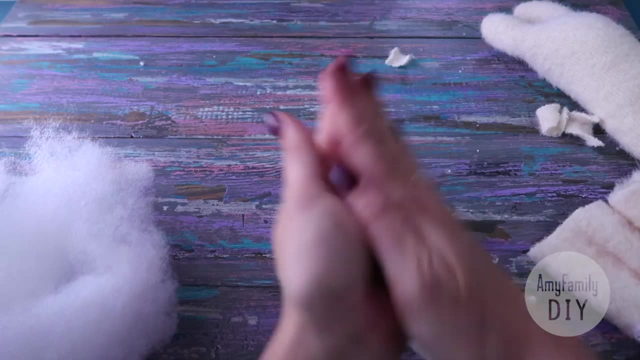 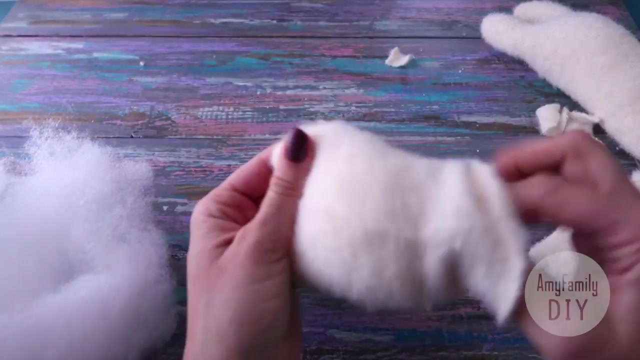 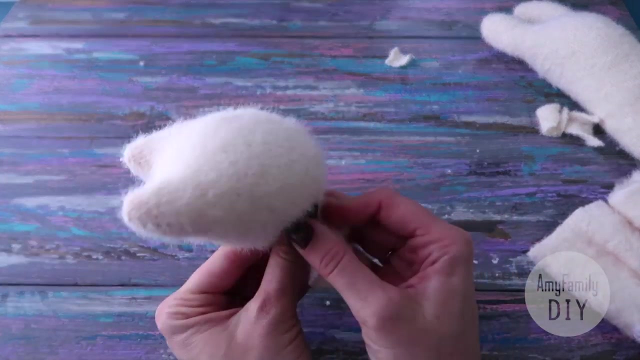 Cut off the excessive part of the sock and turn my piece inside out. First I stuff the ears with small balls of hollow fiber, then stuff the rest of the head, Then just stop. Good, Ok, It's done. Let's see how it matches the body. 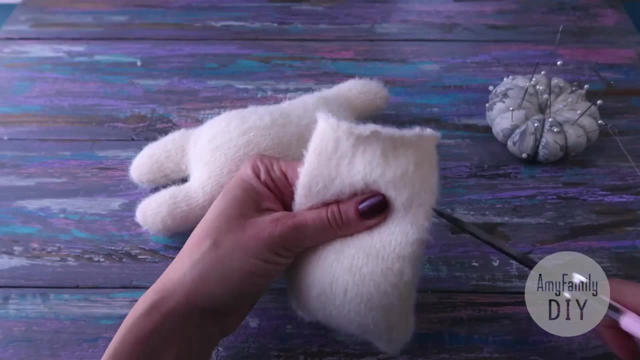 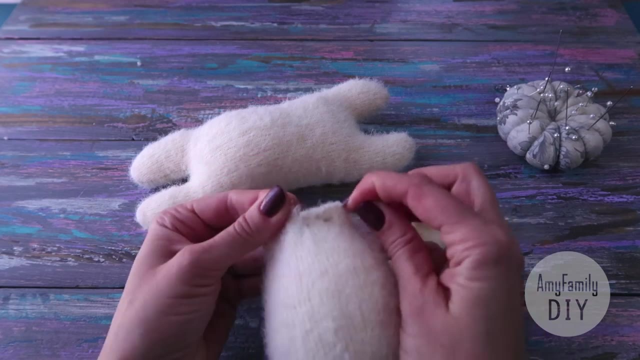 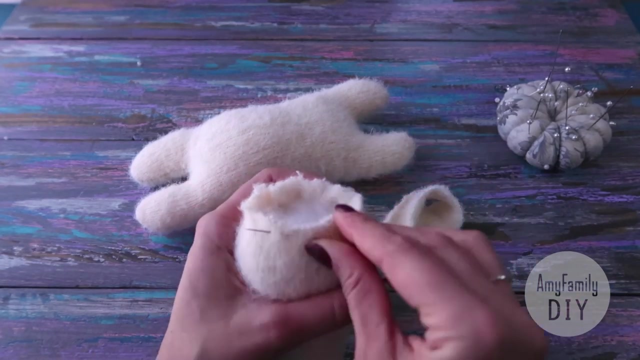 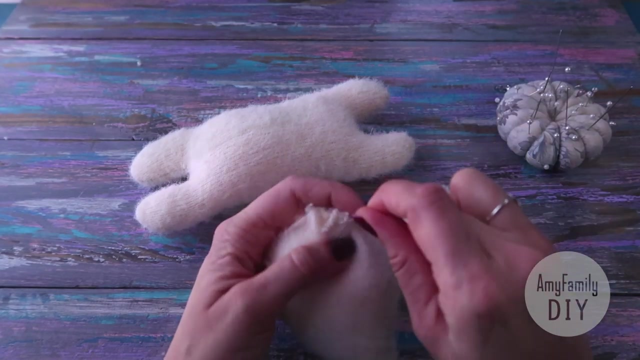 Looks amazing. To sew up the head. I cut off the unnecessary part of the sock, gather the piece together along the perimeter like this and pull the thread. In case of the purple kitten, I've left a longer edge, gathered it together and hid. 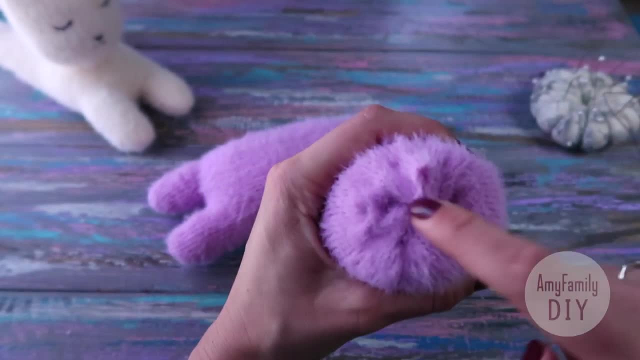 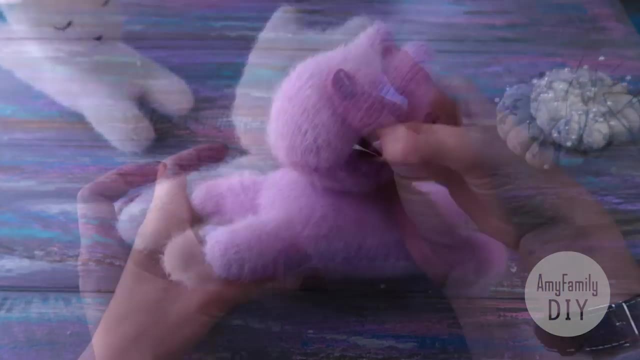 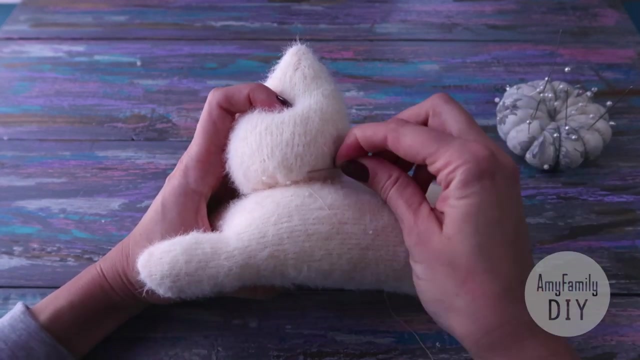 the edges inside before pulling by the thread. It came out very neat. I guess I'll stick to that. Join the head and the body together, Sew around the head. alternatively, running the needle through the fabric on the body and on the head. 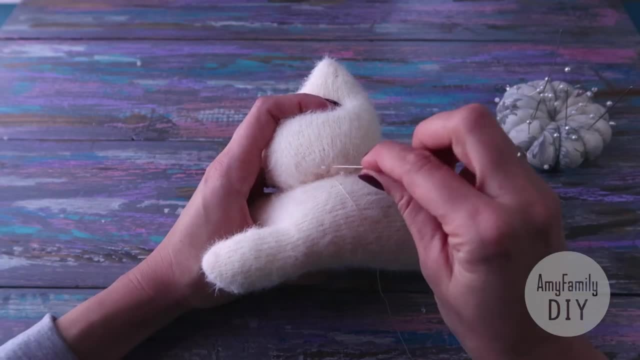 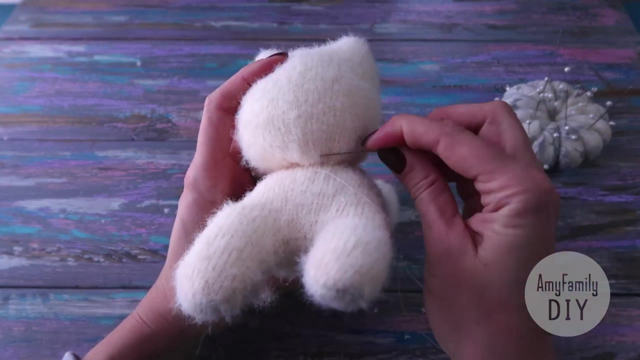 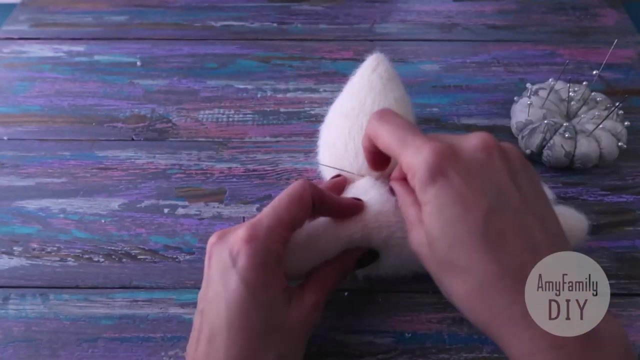 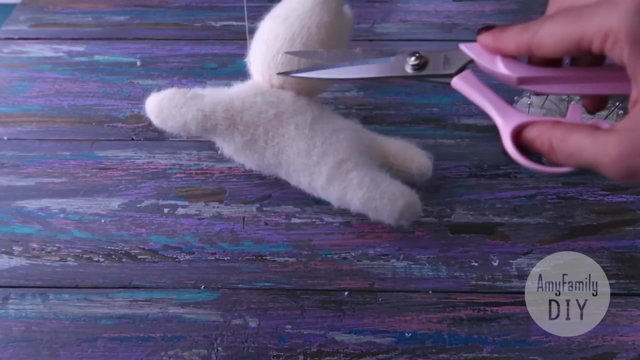 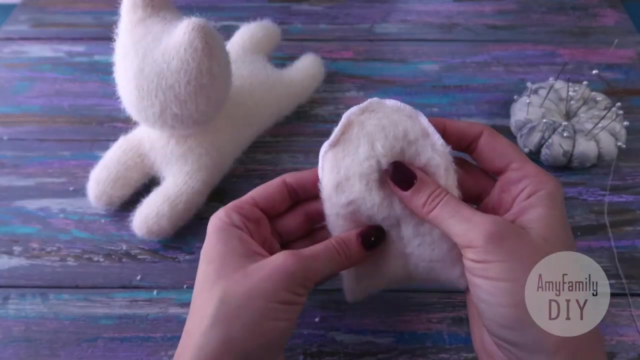 You can make a few circles like this. At the end I tie a knot And hide the thread inside the toy Like this. Now cut it off. Looks just wonderful. I already imagine how happy my daughter is going to be. And the last but not least, the tail. 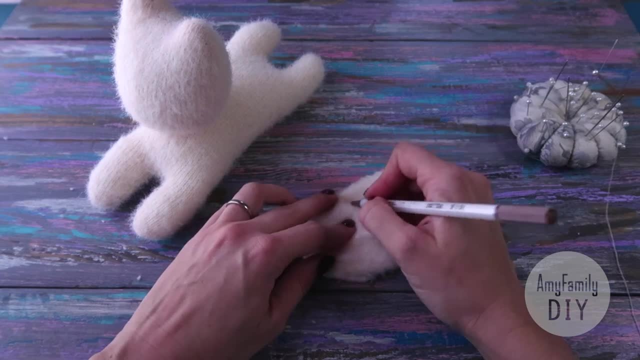 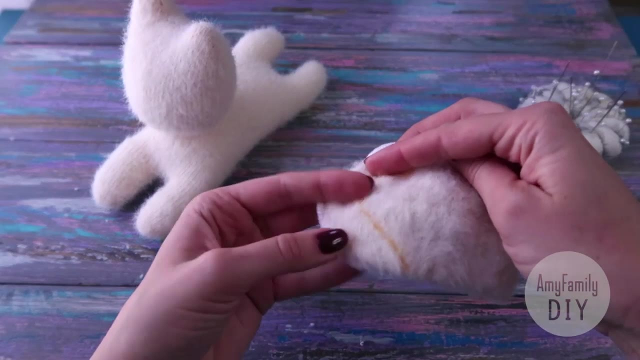 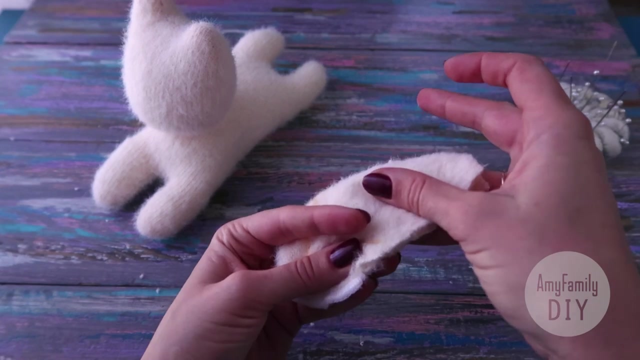 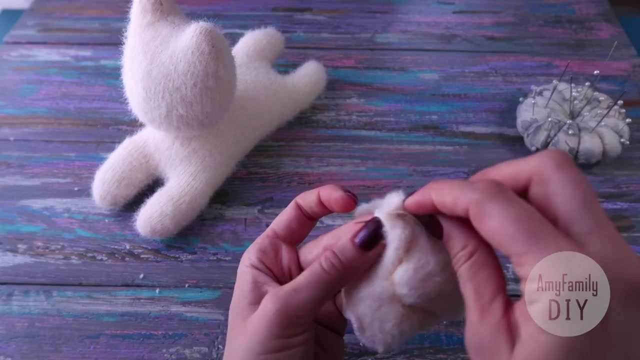 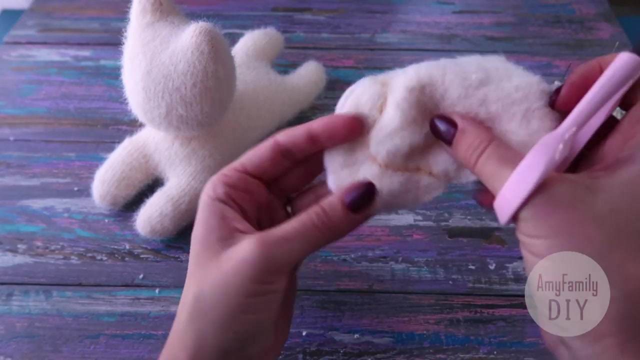 I draw it like this towards the rounding up part of the sock where originally the toes are meant to be At the bottom of the tail. we need a small opening to later turn it inside out. So cut the sock like this: Sew along the line using the backstitch. 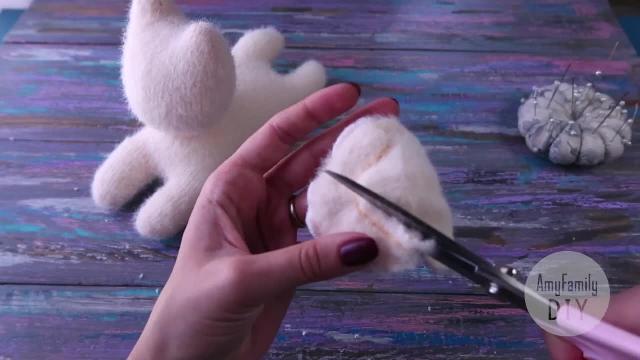 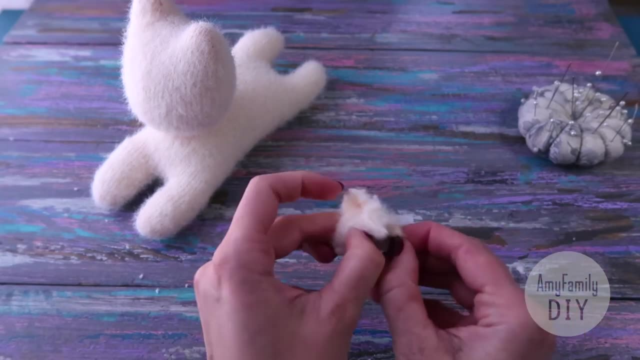 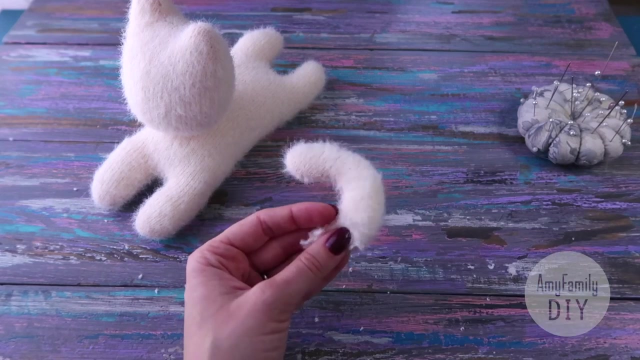 Cut the piece out, leaving half a centimeter allowance, and turn it inside out. It is wonderful, It's nice And it's taught me. I love it Acting. I stuff the tail with holofiber, helping myself with a pen. 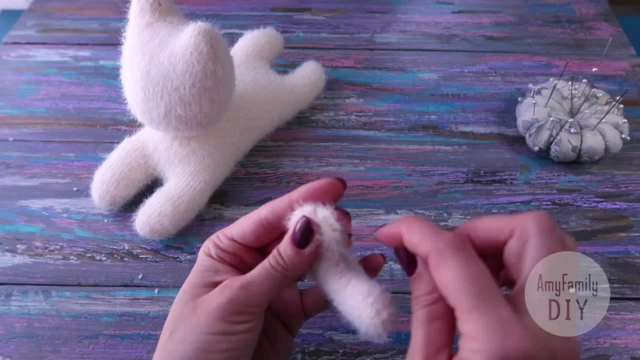 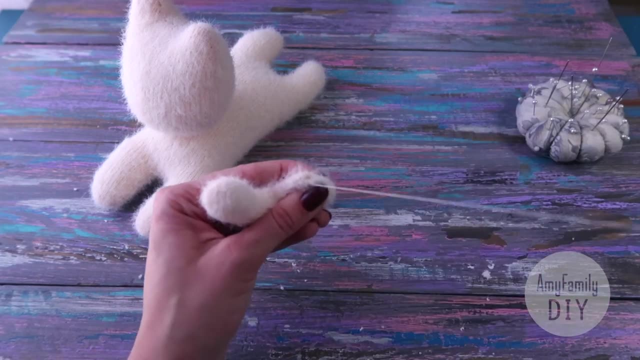 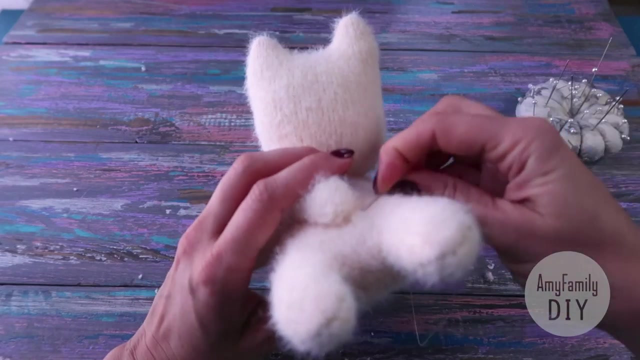 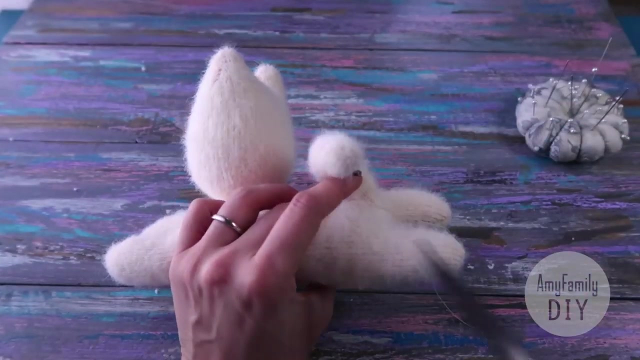 I tuck the edges in and sew up the opening. Now we can attach our tail to the body, Place it like you like it and sew it on. alternatively, running the needle for the tail and the body, Make a few circles like this to make sure it stays in place. 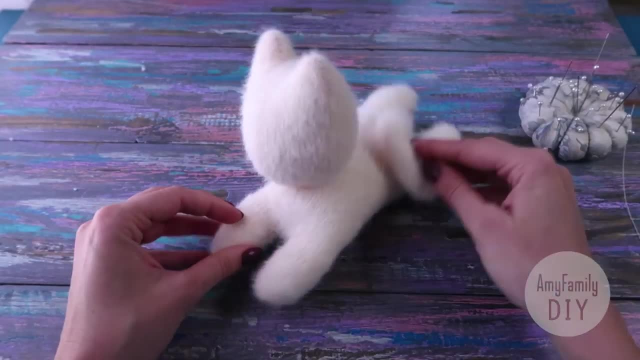 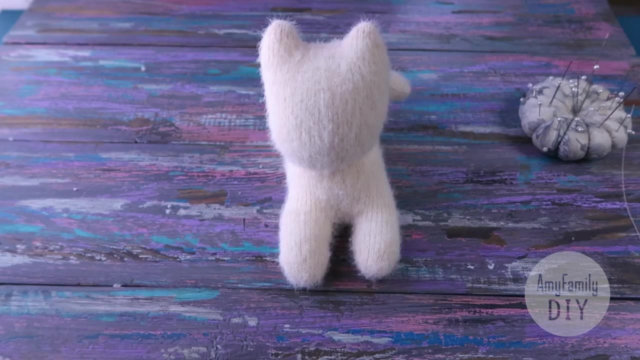 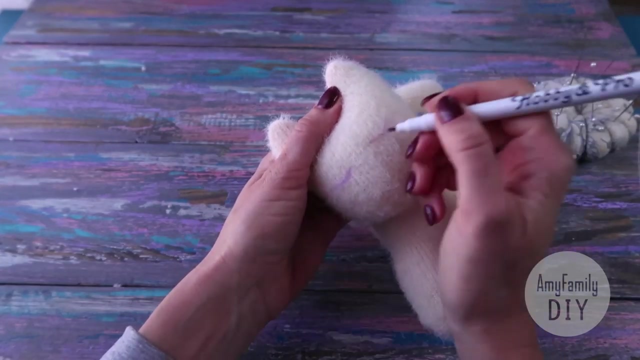 And that's it. my kitten is ready. Now there's just one thing left to do. Let's draw the kitten's face. This little one I imagined with the eyes closed. I draw them with a disappearing pen for tailors. Now I make the stitches along the lines.